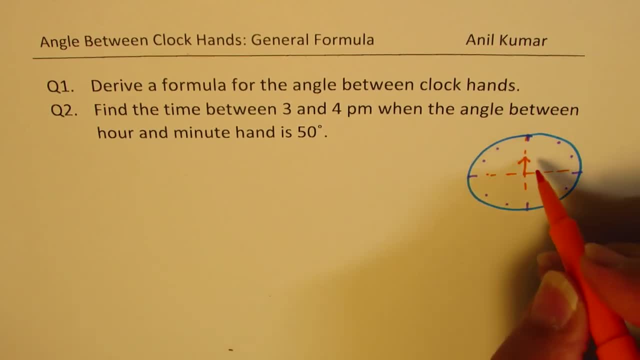 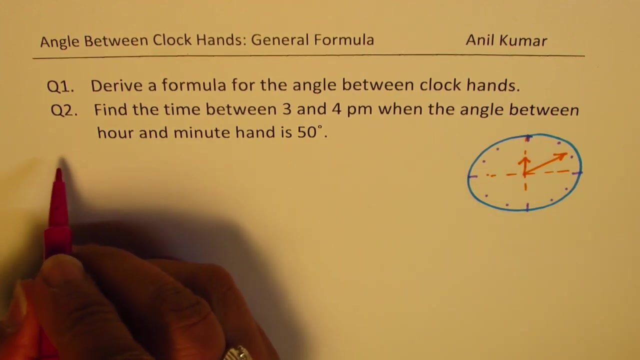 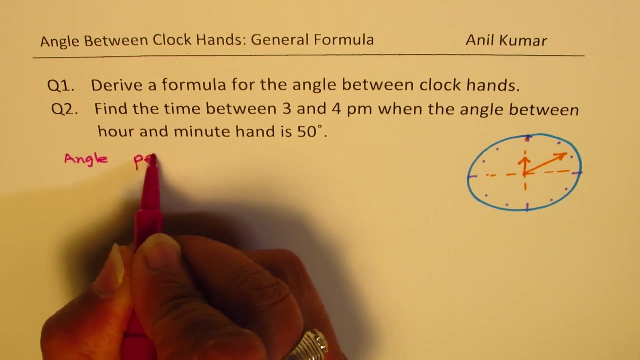 can see there will be an hour hand and there will be a minute hand, correct? Now let's consider both the hands one by one and see how much angle do they cover in a minute. right, That's the point. So we are basically interested in finding angle per minute. That. is the concept? First, let's look at the angle. Let's say 1,, 2,, 3,, 4,, 5,, 6,, 7,, 8,, 9,, 10,, 11,, 12.. Let's say 1,, 2,, 3,, 4,, 5,, 6,, 7,, 8,, 9,, 10,, 11,, 12.. Let's say 1,, 2,, 3,, 4,, 5,, 6,, 7,, 10,, 11,, 12.. Let's 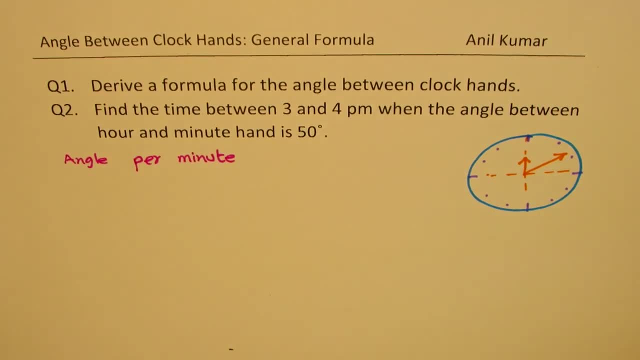 first let's begin with the hour hand, right? So let's see do our calculations for the hour hand. So as far as the hour hand is concerned, there are 12 hours and it goes through 360 degrees In one hour. it will go to 360 divided by 12.. That makes it 30. 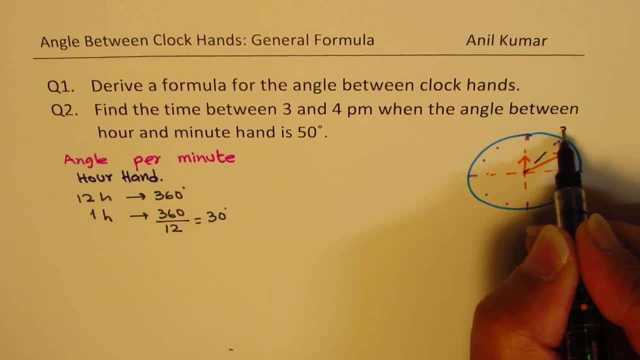 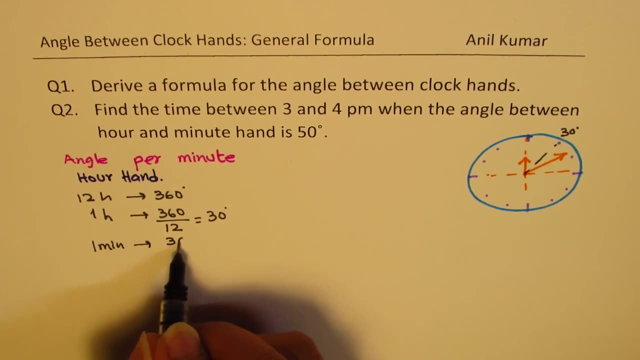 degrees, It makes sense. So that much is 30 degrees, Correct. And in one minute it will go to 30 degrees divided by 60, right, So half a degree. So as far as the hour hand is concerned, it moves half degree every minute. Now let's 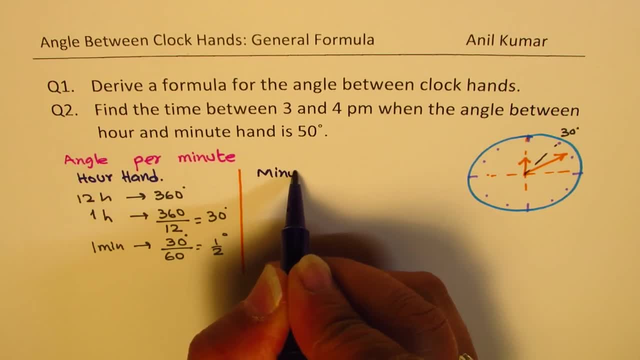 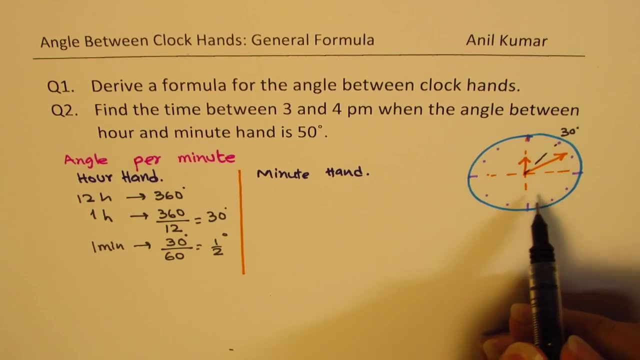 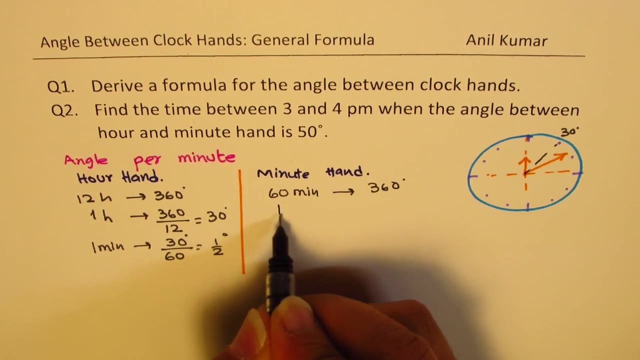 do the same calculation for the minute hand, right? So when we look into the minutes, in all there are 60 minutes and 360 degrees. One minute will be 360 degrees divided by 60. So one minute gives us 6 degrees, right? So definitely, since we have a difference. 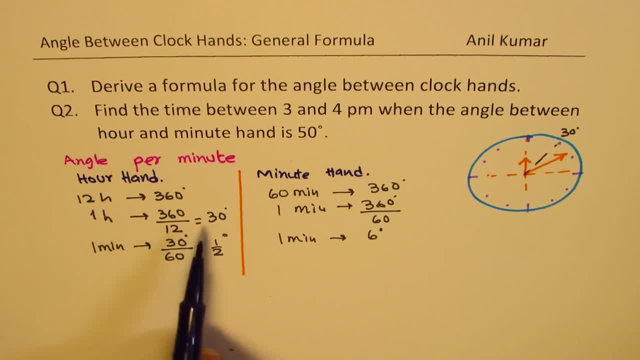 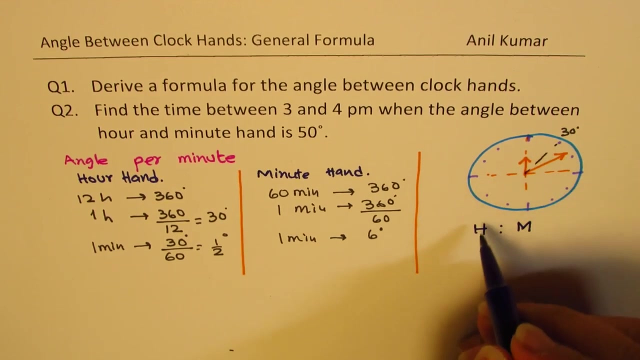 here in the movement, our hand gives in one minute, half degree and as far as the minutes hand is concerned, gives you six degrees. okay, now let's also look into the time right. so normally we say time in hours. let's say some hours and some minutes. now, when i say hours every hour, the hour hand will give you 30 times hour. 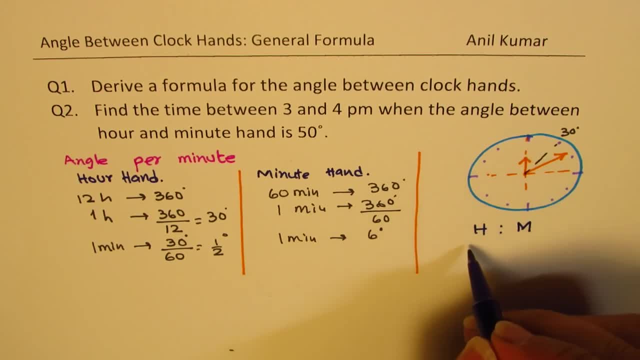 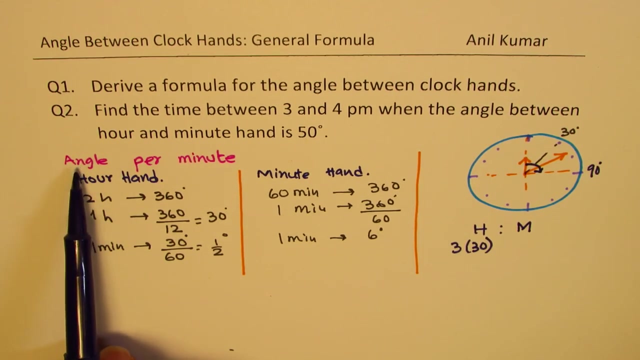 does it make sense 30 times hour? so if it is like, let's say the if i go for three hours in three hours the hour hand moves three times 30, which is 90 degrees, does make sense. so now, as far as the movement is concerned, if i have time which is in hours and 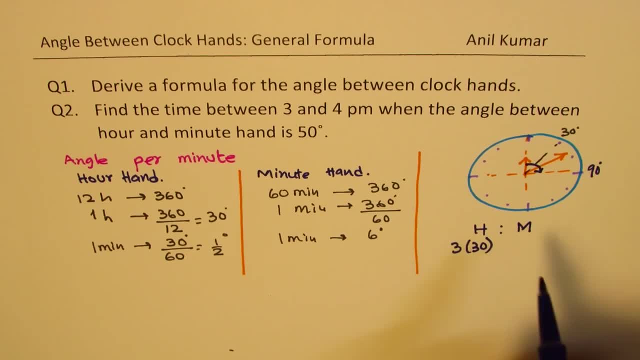 minutes. then in that case, let's say we have three hours- in that case the minute hand will go three circles, do you see? so it'd be like three times 360, but basically it comes to zero. so for a whole number of hour, minute is zero because again starts from zero. 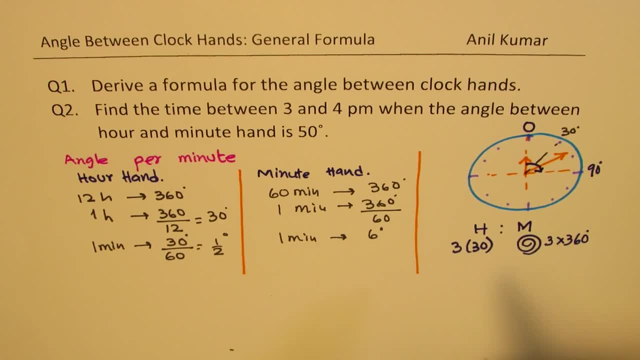 do you see that right? so in general, if we have time in hours and minutes, our hand moves. how much our hand moves? number of hours times 30, 30 times number of hours h plus. for every minute it moves half a degree. so it is half of m. so that is the movement of the overhand. 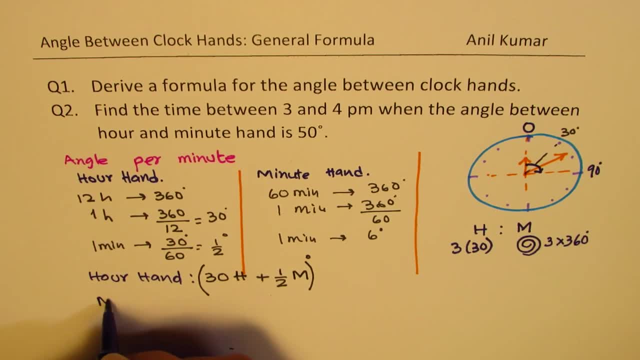 correct for minute hands. this is 6 degrees per minute, so we can write 6 m in degrees. perfect, now we know this. what is the difference? difference gives us the angle between them. let's say angle theta is what that difference will be: 30 h plus half of m, minus 6 of m, right? 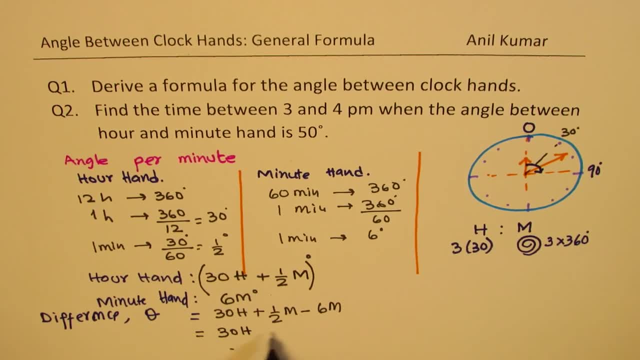 perfect, and that gives you 30 h plus. you can write like this: to 1 minus 12 m, which is 11, right? so that gives you the formula that theta. the angle between them is 30 times hours. 1 minus 12 is minus 11 by 12 minutes. so that is the angle, theta. so a general. 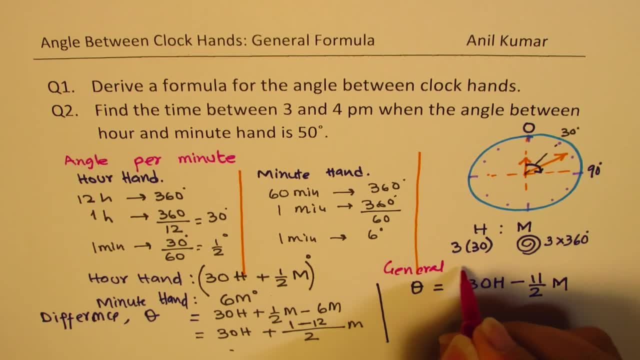 formula here is theta. is that much now? theta should always be positive and therefore we always take an absolute value. so theta is always taken as positive because the minutes we did hours minus minutes position, but the minute's position could be on either side of the hour's hand right, so it has to be positive. 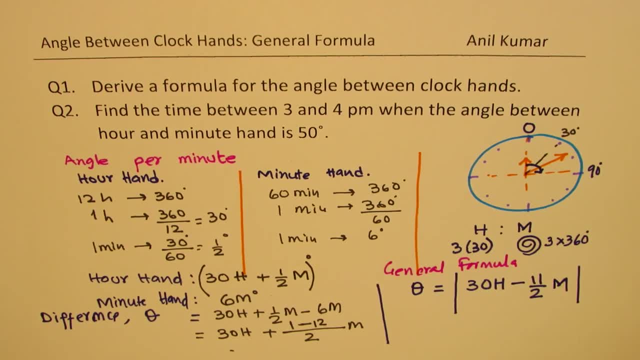 right. so that is the angle theta. is that much right now. that part will be very clear when we do the second question, right? so i hope you got an idea of how to derive the general formula. so the angle moved by the hour's hand is 30 times the hours plus half for every minute. 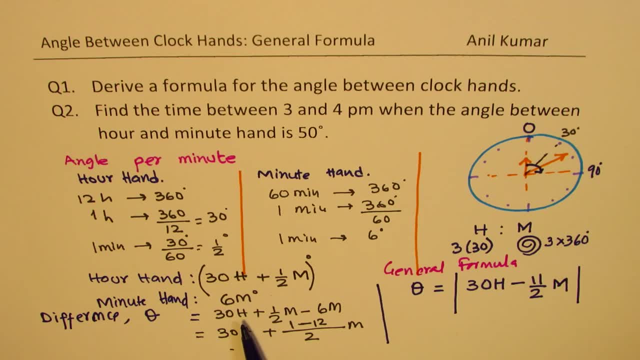 angle moved by the minute's hand is: as far as the hours are concerned, it makes zero, since it goes full circles and for every minute it goes six degrees per minute. so their difference gives us the angle between the two right. so angle between the two is given by this formula clear. 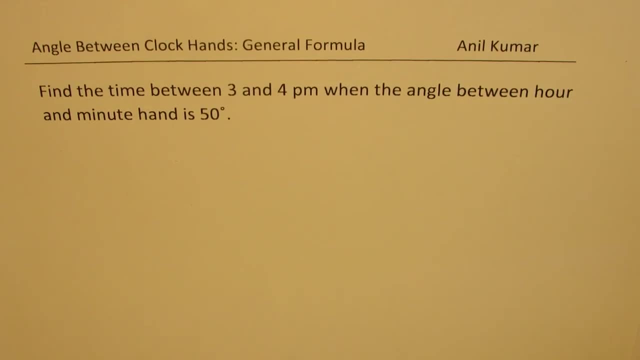 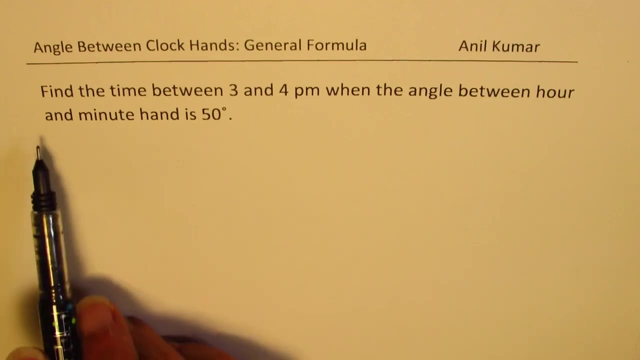 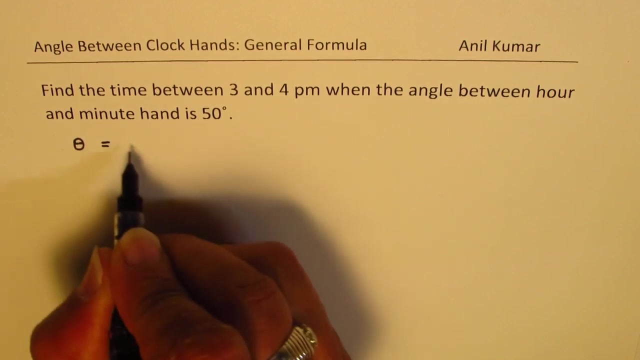 now from here let's go to question number two. the question number two is: find the time between three and four pm when the angle between the hour and the minute hand is 50 degrees. so we just derived a formula saying theta the angle between them is absolute value of. 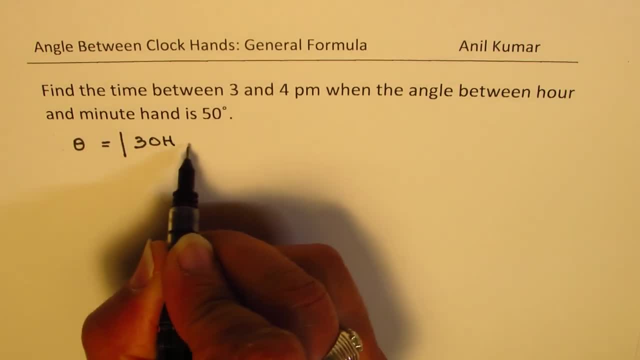 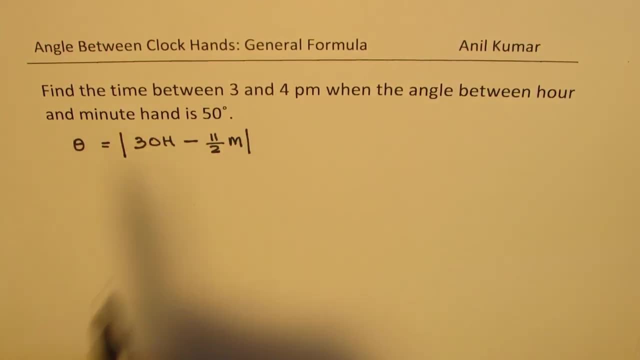 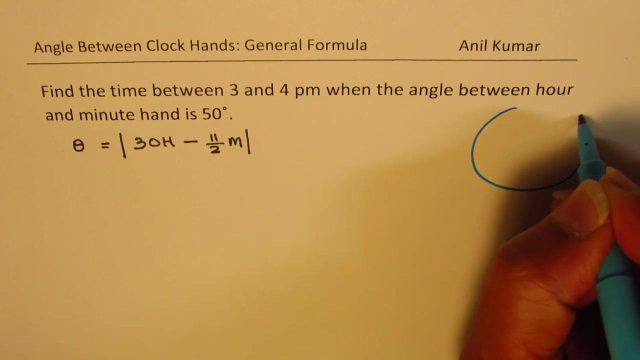 30 per hour, right minus 11 by 2 per minute. so that is it. now we are looking for time between 3 and 4. that is to say, let's sketch the scenario right. so let's say this is 12, 6, 9, 3. so when we say between 3 to 4, that means the. let's say: 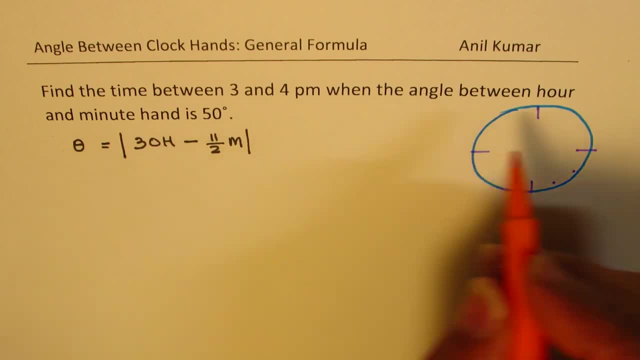 this is 4 and this is 5. that means the our arm is somewhere between 3 and 4, right, so it could be, let's say here: okay, so in that case the minute sum could be somewhere there, right, giving you 50 degrees angle. or we could have a scenario where the the hour arm. let me make minute. 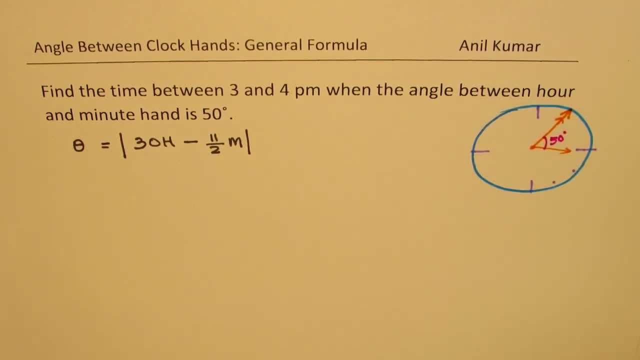 sum longer. okay, okay, that's making sense. or we could have a scenario something like this and 50 could be something like this. so there are two different scenarios. perfect minutes could be before hour or after, and there could be 50 degrees angle between the two when the our hand is between the position three and four. 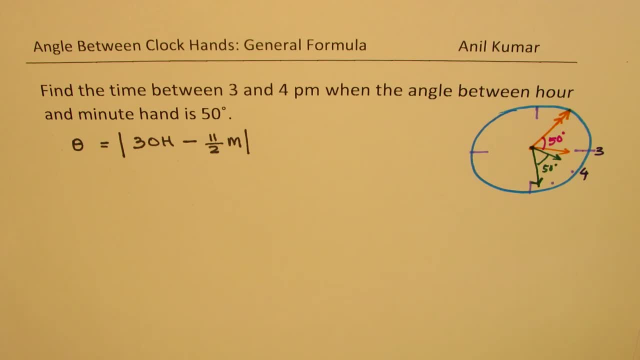 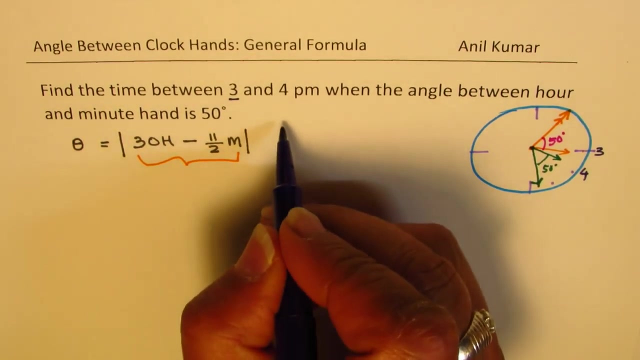 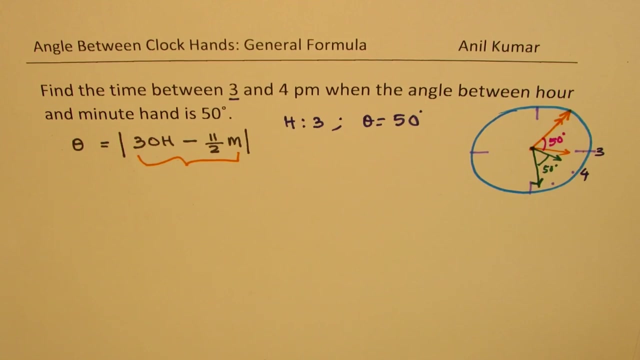 is that clear, right? so basically, what we are saying here is that this portion here is equal to minus theta or plus theta. perfect, now in our case, we are looking into after three, right? so? so the hours will be three and we are given theta as 50 degrees, so we'll substitute and find minutes. 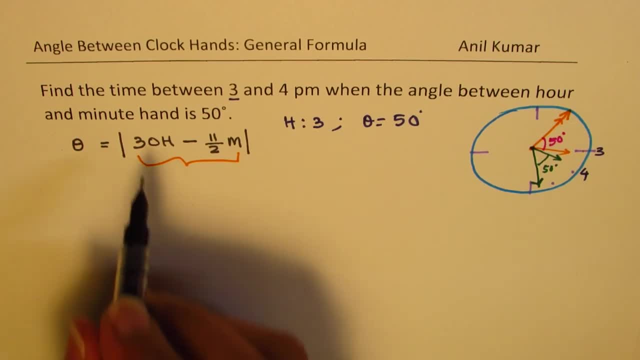 that's the whole idea, right? so we have two equations to work with. so the first one here is that we have 50, which is absolute value of 30 times 3 minus half 11 over 2 of m, right? so that is, we could write this as 50. 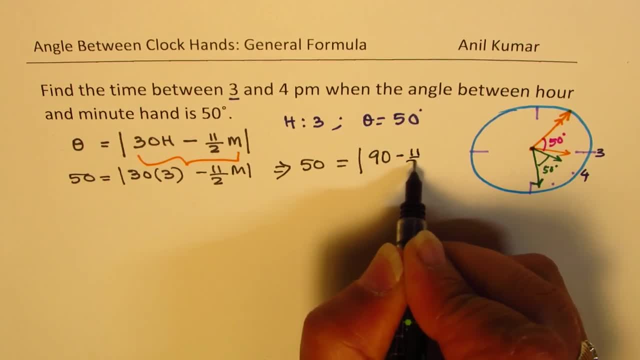 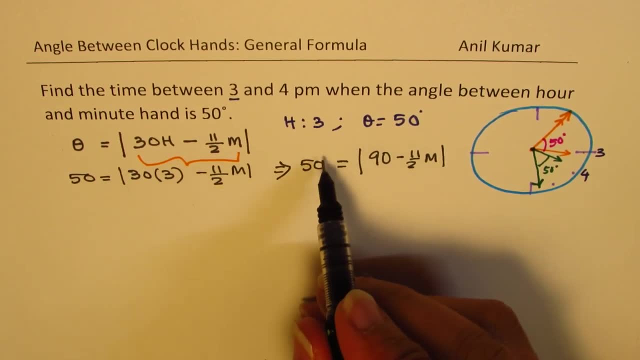 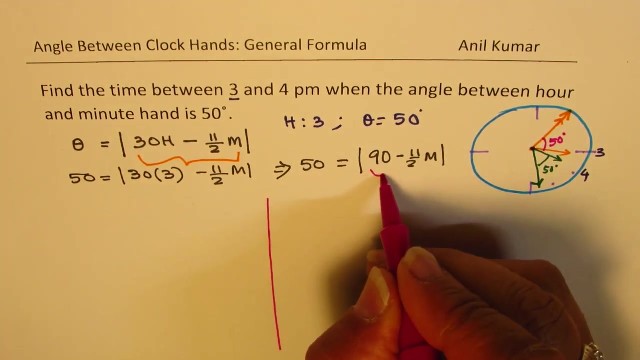 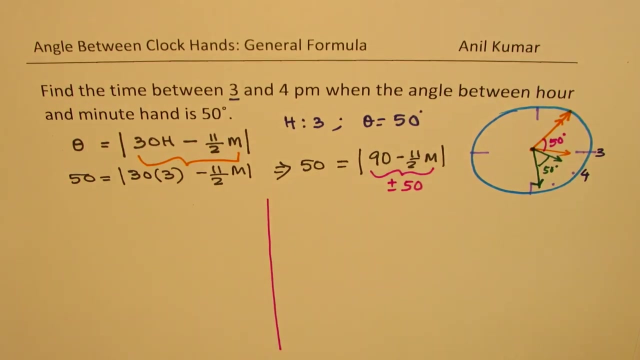 equals 2. absolute value of 90 minus 11 over 2 m. perfect. this is in degrees, right, so we get 50. degrees is equal to minus 50. that's what we all fantasy of ten times better. so this is the вход point here. this is one of the inputs, the example input, the out wrap: overant Saud. 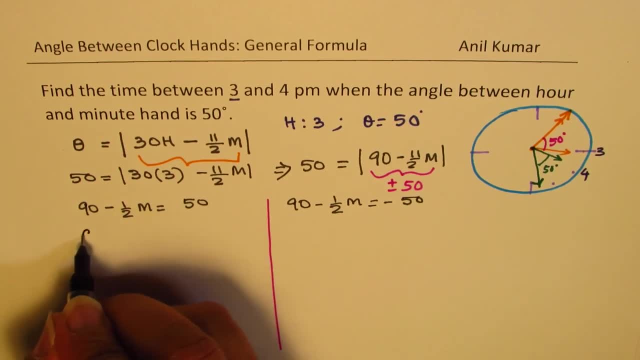 so today we are going to solve dagger. in this particular case, xiong only wins. and when we solve the deduction of for I f also ins, translating, we get 90 minus 50 equals to sorry 11 over 2m, sorry 11 over 2, 11 over 2m, and that is 40. 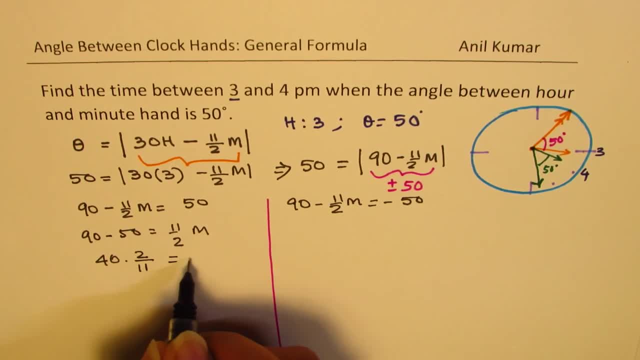 times 2 over 11 is in minutes, correct. So that is, let's multiply 80 over 11 in minutes. So dividing we get what 7 times and then 3 over 11, correct, So those many minutes. 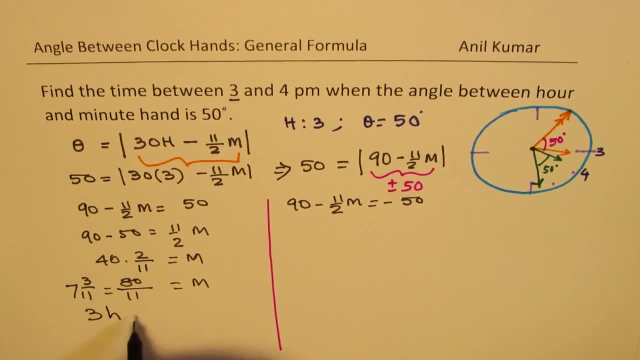 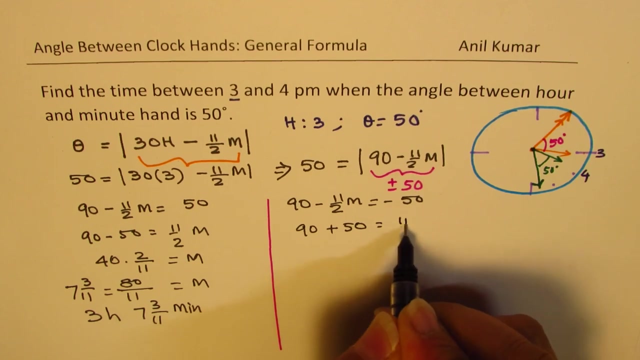 So we have here 3 hours and 7,, 3 over 11 minutes. Is that okay? So that is between 3 and 4, correct. On the other hand, I will do 90 plus 50 equals to 11 over 2m, that is. 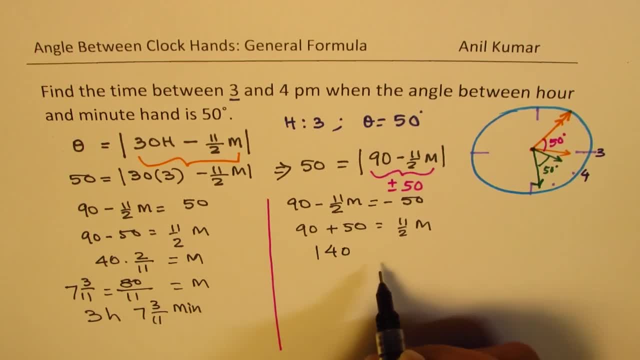 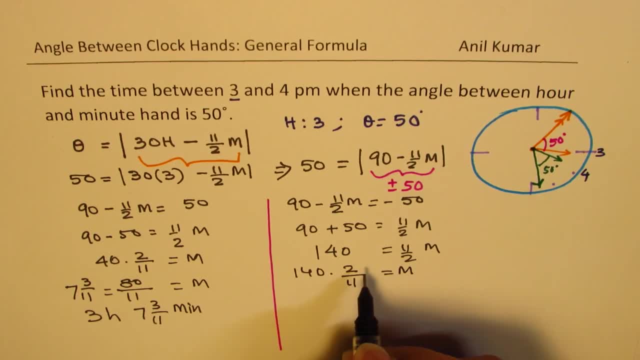 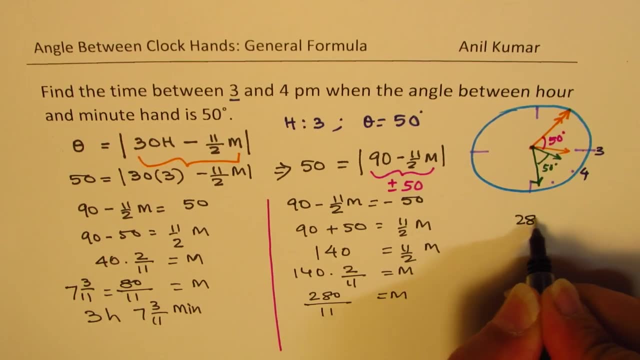 times 2 over 11 is M, so we get 280 divided by 11 is M, so you could divide 280 by 11. okay, so we get two times, which is 22, and then we have 60, so five times is 55. remainder is: 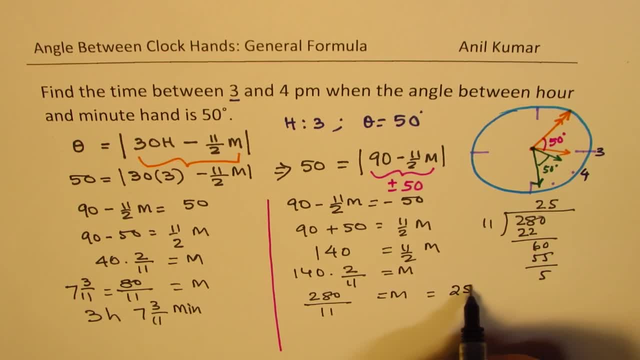 five, so we get 25 minutes and 5 over 11 minutes, correct? so the other answer for us could be here: three hours and 25, 5 over 11 minutes. is that you? so that is how we can get two different answers as kind of a question. so that is how we can get two different answers as kind of a question. 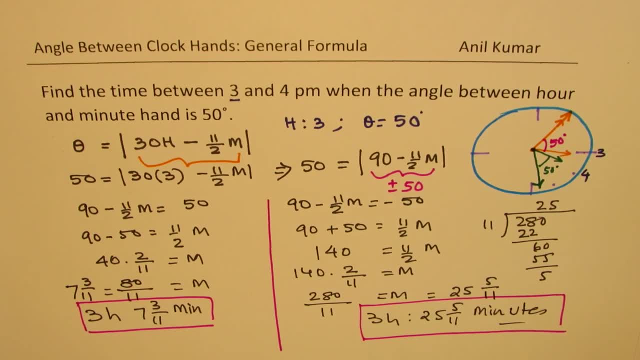 of shown here in the dagger does make sense to you, right? so that is how, knowing the formula, we can I easily solve this question. so it's kind of important to understand how to derive the formula and apply it now. once you know the form, though, all these questions can easily. 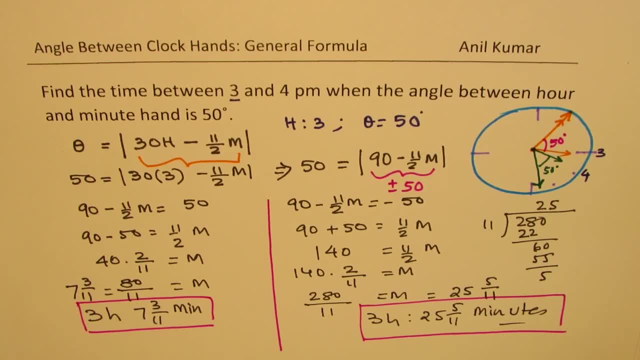 be solved. I hope that makes sense. feel free to write your comment, share your views and, if you like, and subscribe to my videos. that be great. thanks for watching and all the best.